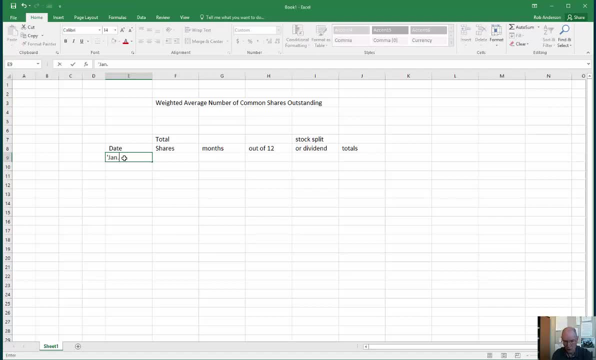 So we start at the beginning. We start at the beginning of the year with a certain number of shares. So once again, let's start with 500,000.. And the question is: how many months do we have 500,000 shares and not more and not less? 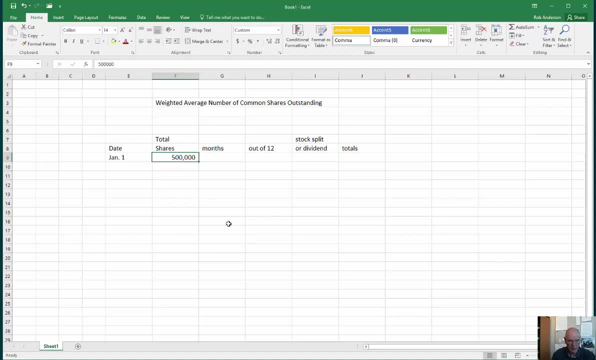 So this, by the way, is common shares outstanding, not preferred, because EPS is only for common shares. So let's just say that on February 28th- not a leap here- I guess we repurchase 40,000.. 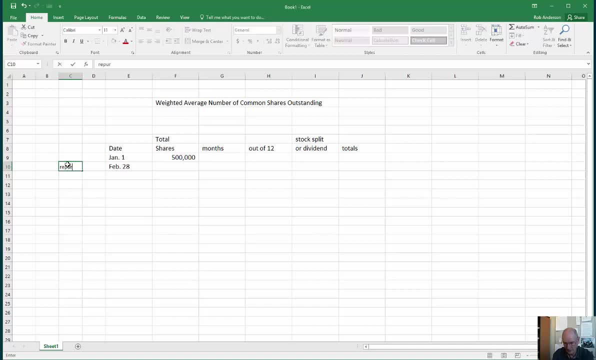 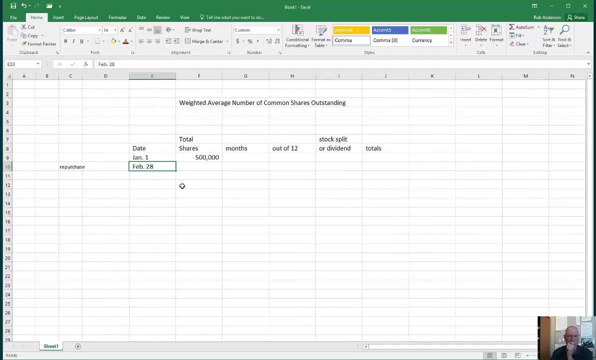 So I'm just going to write this here. That's a repurchase. We just want to make sure we keep track. I should even write it here: We repurchase 40,000.. So the question now is how many shares are outstanding. 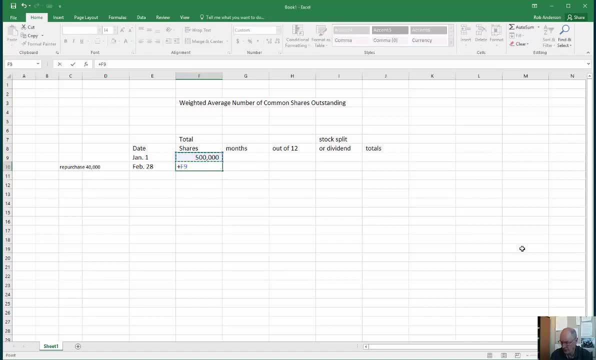 And of course it's 500,000 minus 40,000.. 460.. So now we know there was a share transaction and it went down. So the question now is: for how many months did we have 500,000 shares outstanding? 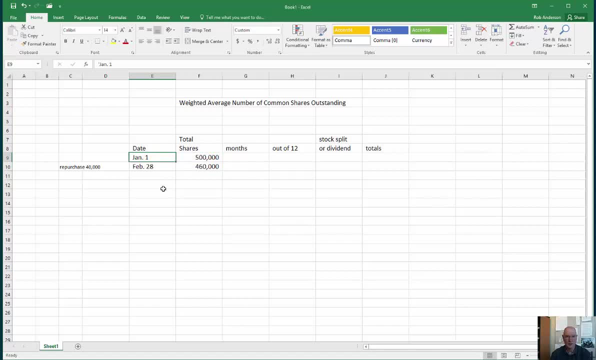 Well, this is all of January and all of February, So to the end of February is when this happened. So two months were outstanding out of 12.. So you have two months out of 12.. Now let's say that along comes. 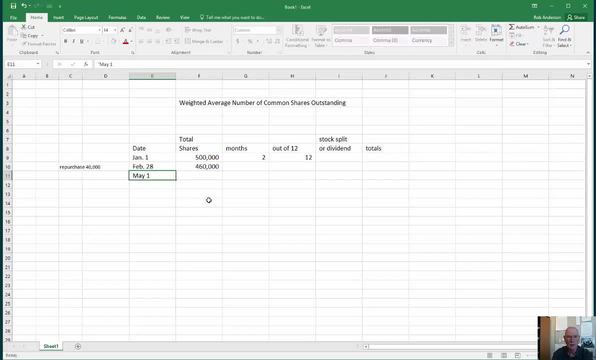 May 1 and we're going to issue 150,000 shares. Now, these numbers are random, Don't worry about it, But here's what happens. We had 460.. So we take the 460 plus 150,000 shares. 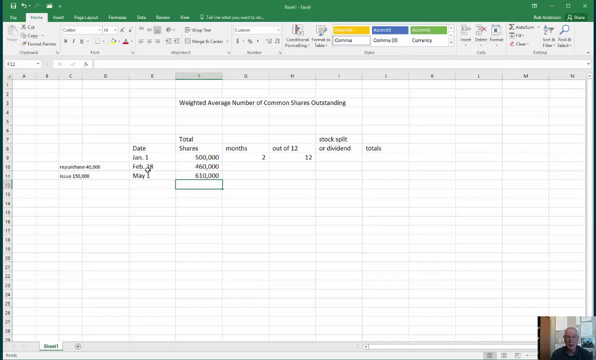 Now we have 610.. We're going to go back here and we're going to say: okay, for how many months did we have 460,000 shares? So this is counting from the end of February. So we're going to go March, April, but not May, right? 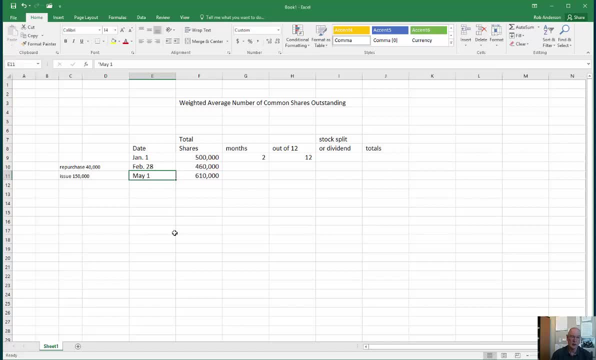 Not May, because this is May 1.. So you have to watch these dates right. End of February to the beginning of May is two months, So once again, two months out of 12.. Two months out of 12.. Okay. 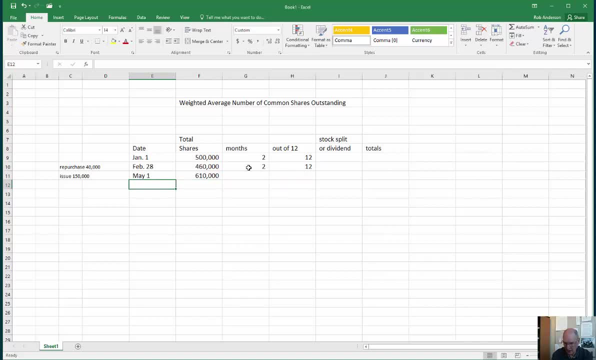 So along comes, let's just say, September 1.. And we're going to have a 241 split. Okay, Now I think you know what that is. A 241 split means we retire the 610,000 shares, And then what we do is we issue twice as many. 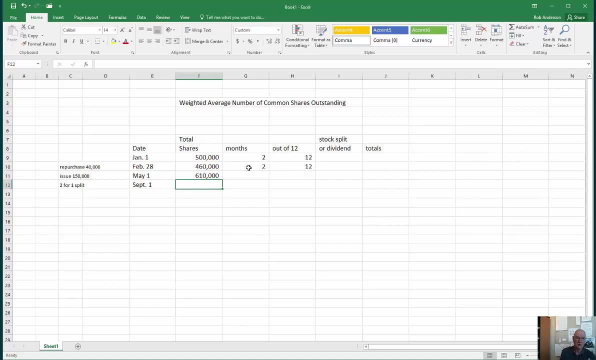 So if a shareholder had 100 shares, we issue them 200 new shares. A company may do this in order to drop the price of their shares, to facilitate a more active market. You know, if you get up into the point where your shares are costing. 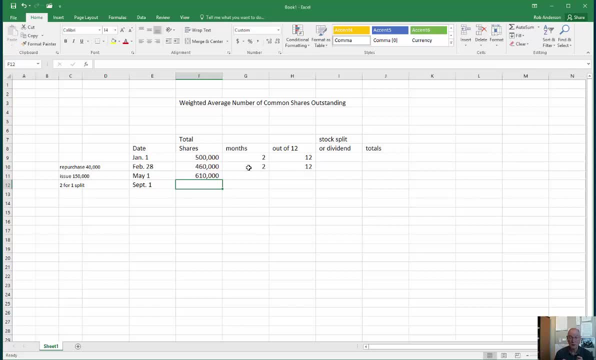 you know, $400,, $500,, $600, it's hard for a lot of investors to buy a block of 100.. So they could do a 2-for-1,, 3-for-1, or even 4-for-1 split. 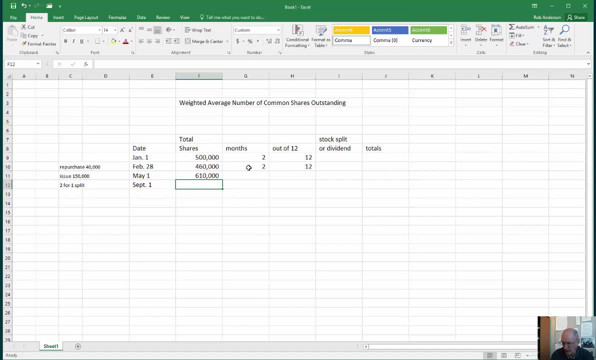 So we did a 2-for-1.. So we're going to have this times 2.. And suddenly we've doubled our shares, right? So we're going to deal with that in a minute. But the question is then: for how many months did we have 610,000 shares? 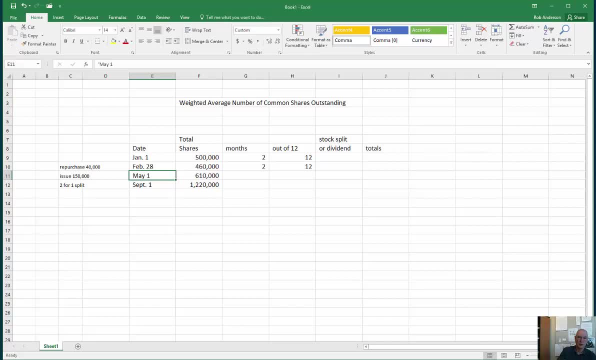 So all of May, June, July and August, So four months. So for four months out of 12, we had 610.. Now last one, Let's just say it's November 30. And we issue 100,000 shares. 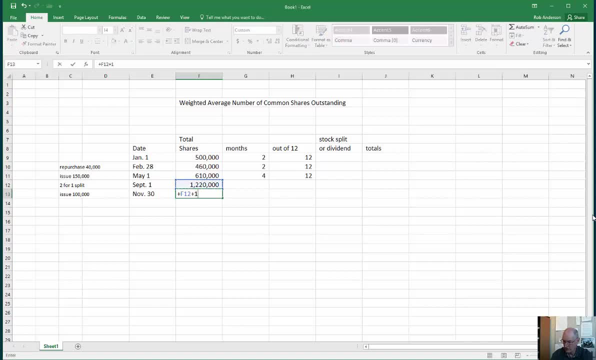 So now we have that many plus the 100,000, 13.2.. So again, let's just go back and say: for how many months did we have 1.22 million shares? So all of September and October and November. 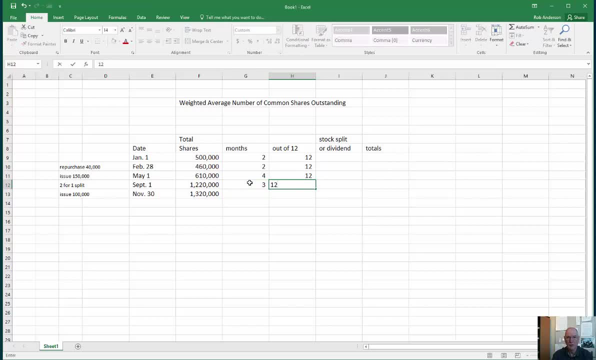 Three months. So three months out of 12.. Now this is it for the year, So we had no more share transactions. So from the end of November to the end of December, one month out of 12.. So we've been really trying hard to count the months right. 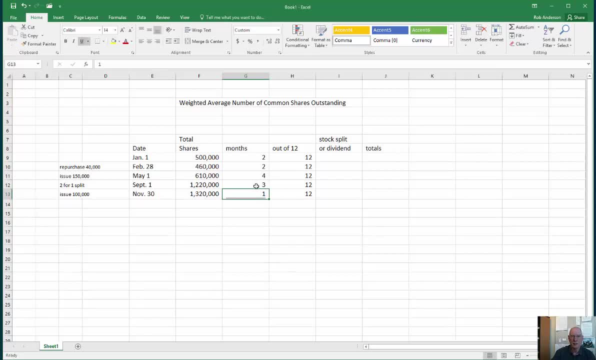 12 months in a year. Let's see if we did it right. I want to add these up and make sure that we really counted 12 months, Because what if we made a mistake here and thought it was five? Well, if we make a mistake here and think it's five, 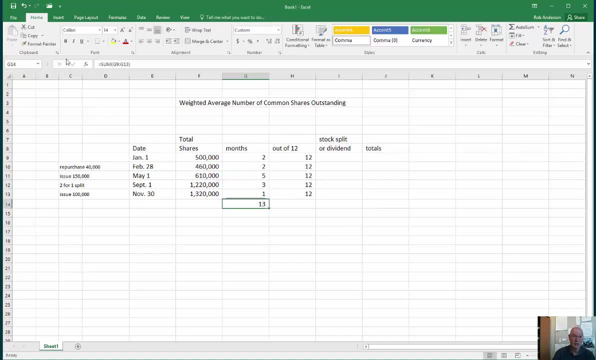 you get 13.. And I go: oh, I made a mistake, Let's put that back. So it adds up to 12.. That's a good sign. Okay, Now one complication. What I'm about to mention is the same for a split as a dividend. 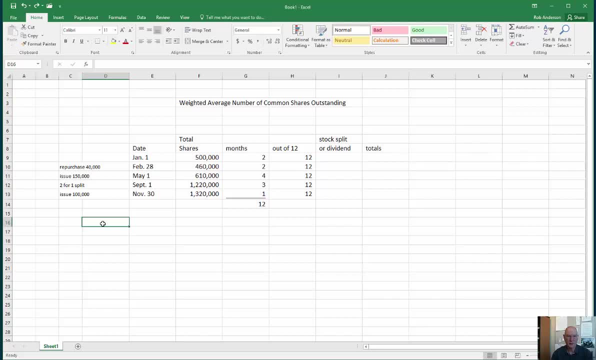 Our weighting is way off now because we didn't actually have any change to our contributed capital, Like here, when we repurchased 40,000 shares. our contributed capital went down Because, as you know, those shares are gone right, You've debited shares. 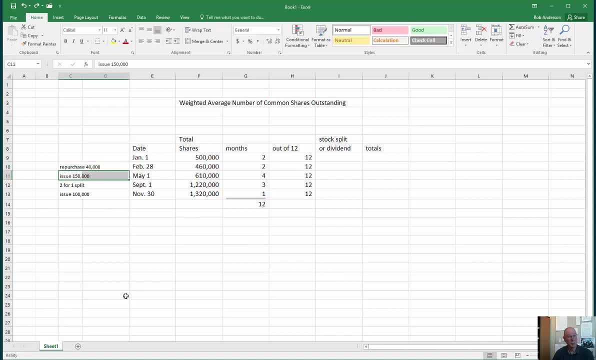 Here, when we issued 150, our contributed capital went up. But here a stock split is just a memo entry, And if it were, let's just say, a 10% dividend, all that happens with a 10% dividend is you transfer the valuation amount. 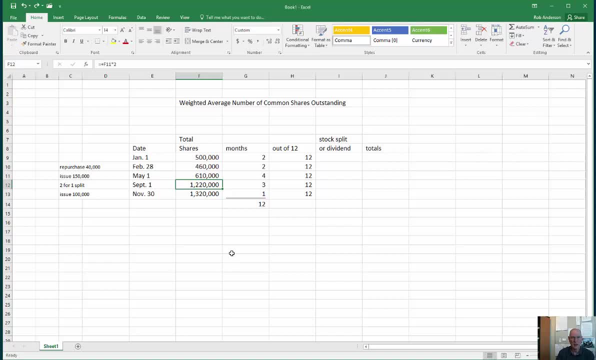 out of retained earnings and put it into your common shares account, So through no change in our capital structure whatsoever. really, in terms of contributed capital we actually have way more shares. So because of that we must restate these earlier amounts, as though the stock split. 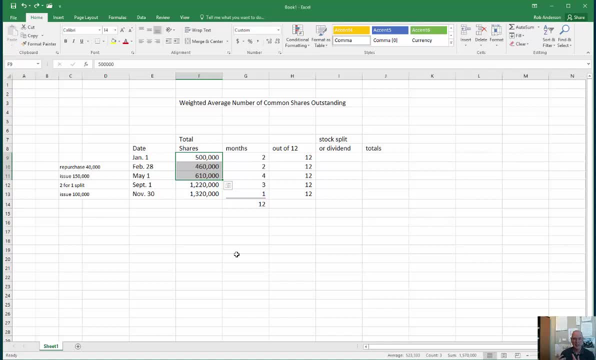 or the stock dividend, had happened at the very beginning of the year And that way everything that we do and all our numbers are representative of having had that split included. So every amount before the split, which again was a two for one split. 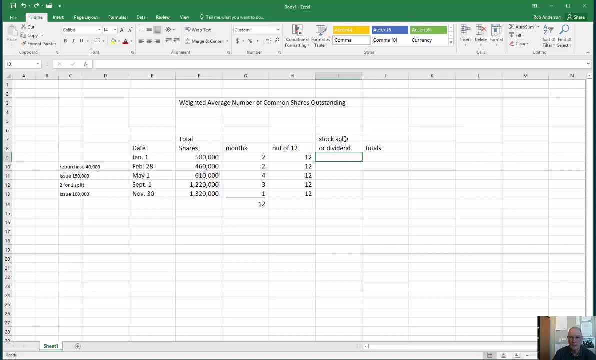 must be multiplied by two. So under my heading here, stock split or dividend, I'm going to put two here and two here and two here. Now there's nothing here because this is including the split. Now I'm going to put this back. 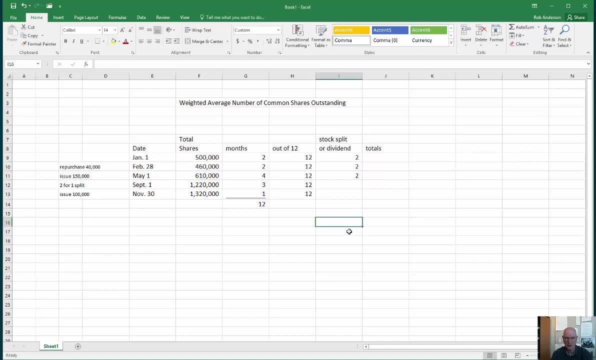 but I just want to mention: if this had been instead, let's say, a 10% stock dividend, then here's what we would do: We would take this and, instead of putting two here for a 10% stock dividend, we would take this. 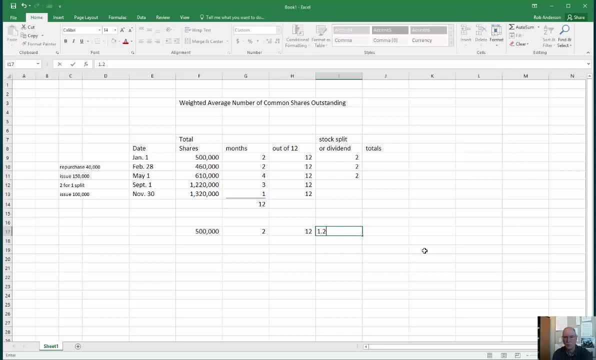 and we would multiply by 1.2.. Okay, so I'll just make that. put the decimal in there. 1.2 works like this. Sorry, did I say 10%? Excuse me 1.1.. 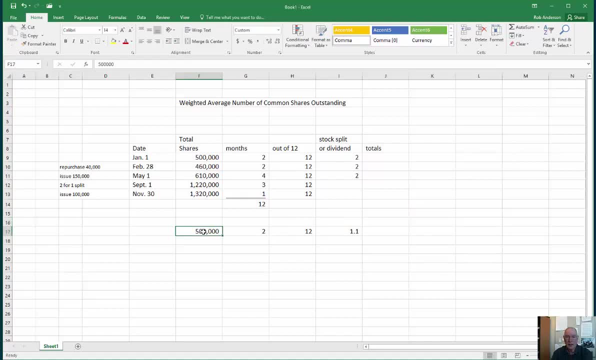 Okay, so the 500,000 is still there And the 0.1 times 500,000 is another 50, right, So by using 1.1, we just save ourselves a math step, but I would do 500,000. 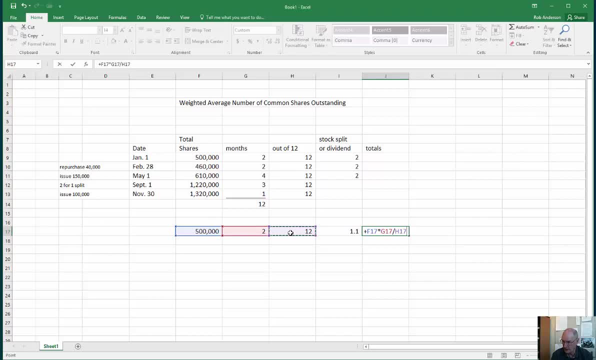 times two months, divided by 12 months, times essentially itself plus the 10%, And this is what we would get Now. remember it's not going to say 550, because this is only for two months out of ten. This is for 12.. 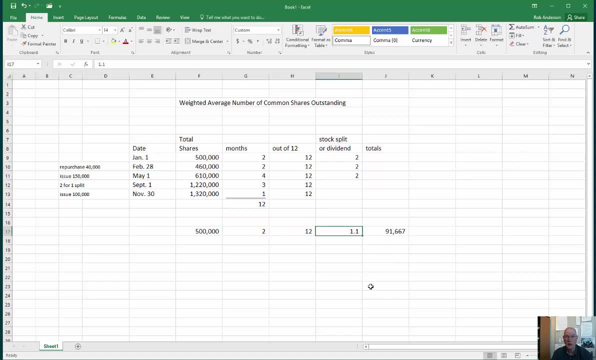 So I'm just showing you this to say this is what we would do if that had been a stock dividend instead of a split. Now it's not, It was a dividend, But we're going to do the same thing now. This gives us double the shares.